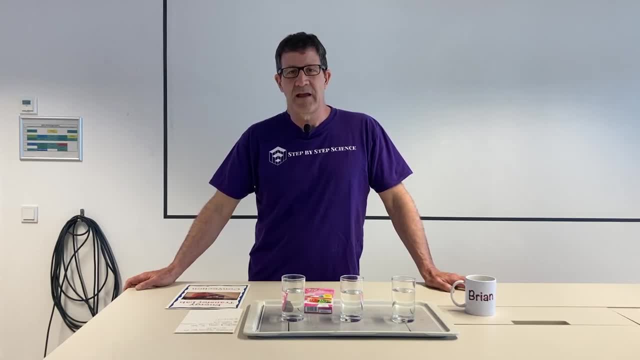 Welcome to the next video in our Making You The Scientist series. Today we're going to do a fun, easy to do lab experiment that's going to demonstrate to you the principles of energy transfer, heat and convection. And this lab is easy to do because all you need is a few materials. 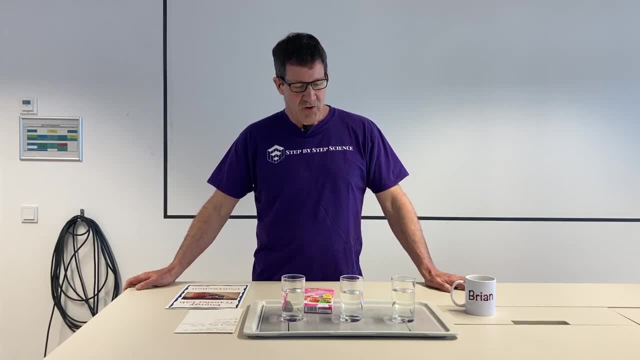 which you probably have in your classroom or even at home. You need three glasses: one with cold water, one with room temperature water and one with hot water, And then the next thing you're going to need is some food coloring. That's really all you need to do this lab. 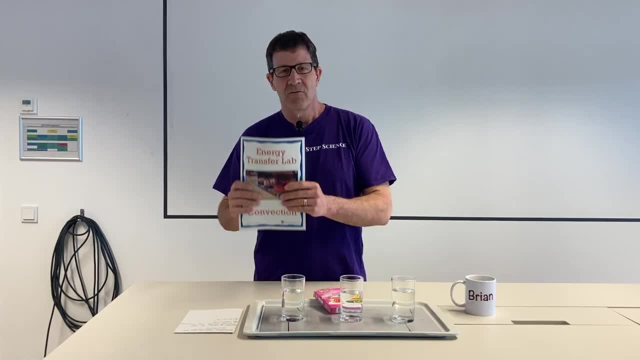 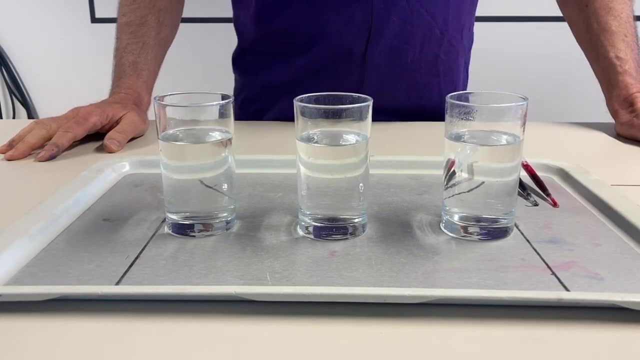 If you would like some more information about this lab, we have a full write-up which is available at our website. The link is in the description below. Okay, now we're ready to do our experiment And you can see here we have three glasses. 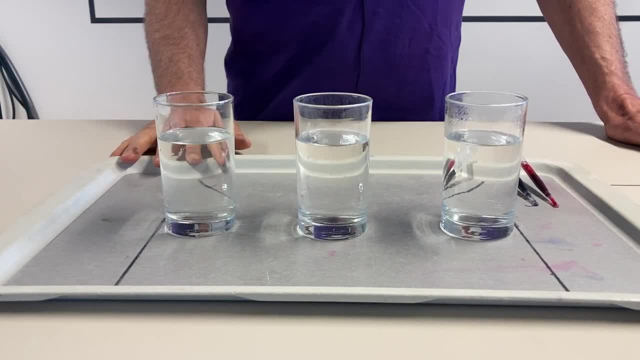 one, two and three, And the water temperature is different in each of the glasses. One of the glasses has cold water, one of the glasses has room temperature water and one of the glasses has hot water. Now, I'm not going to tell you ahead of time which one. 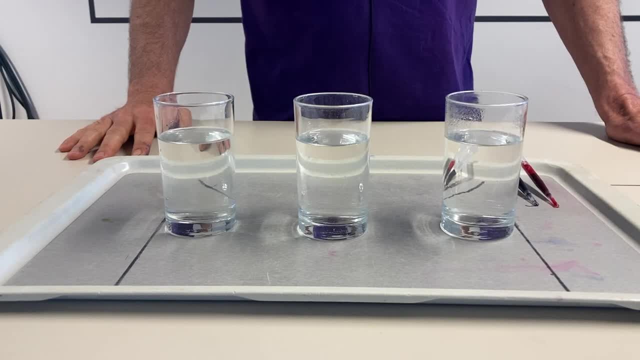 of the glasses has cold water, One of the glasses has room temperature water and one of the glasses has room temperature water. We are going to try and see if we can figure out which temperature is in which glass, based on how the food coloring is dispersed through each of the glasses. Now, 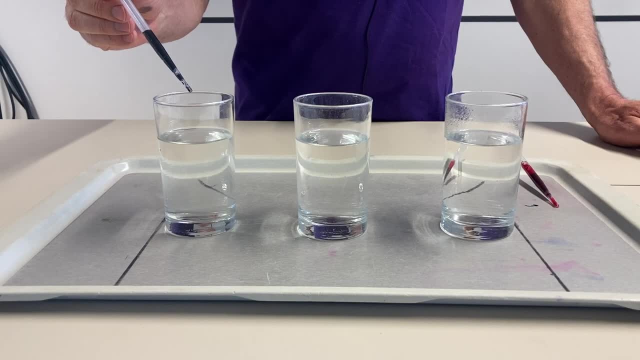 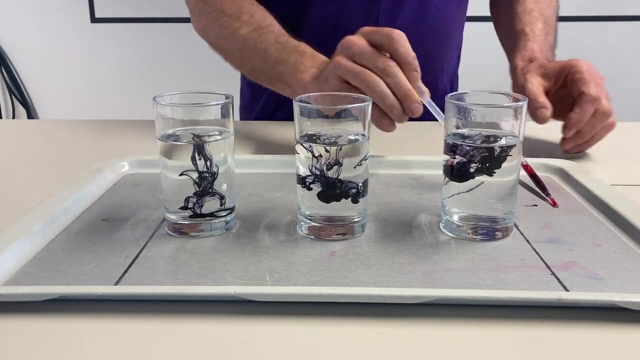 I have blue food coloring and red food coloring and I'm going to put a couple of drops of each color in each glass and we'll see what happens. You can see, as we put that in, the food coloring is being dispersed. It's spreading out through each of the glasses and we want to be able to. 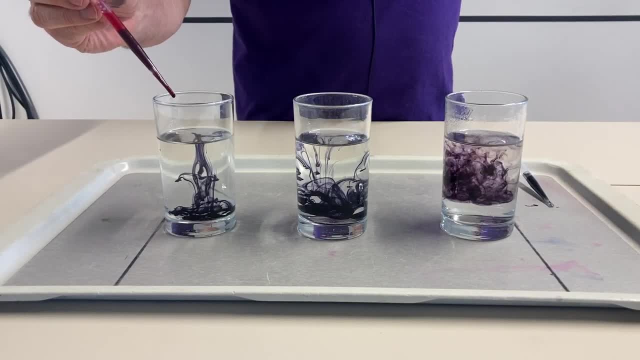 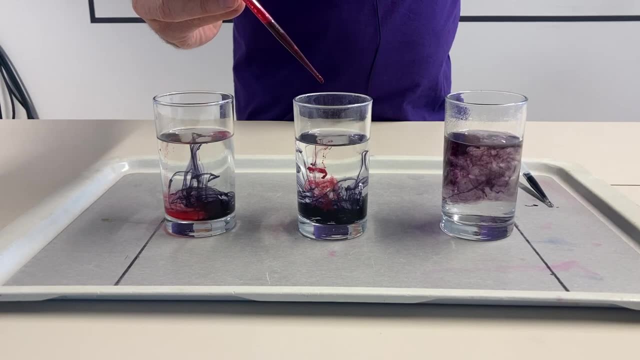 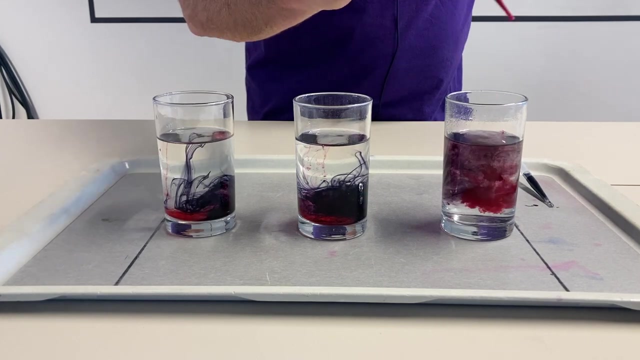 you want your students to be able to make a conclusion based on how the food coloring spreads, what the temperature is in each of the beakers and how that represents the motion of the molecules in each glass. Now, let's just let that sit for a second. All right, now we look at the results of 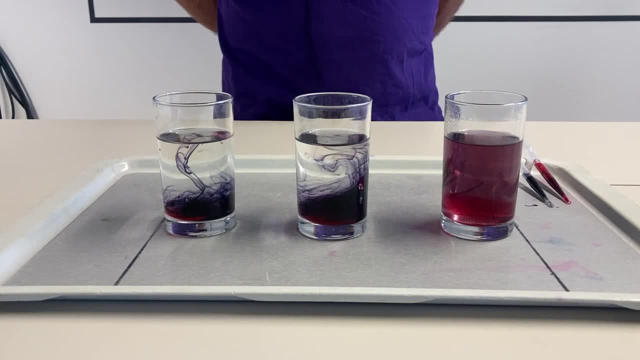 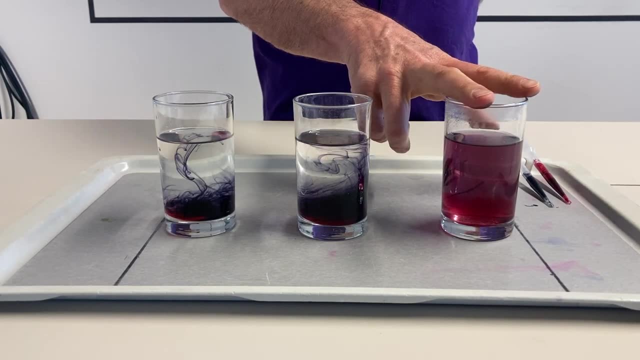 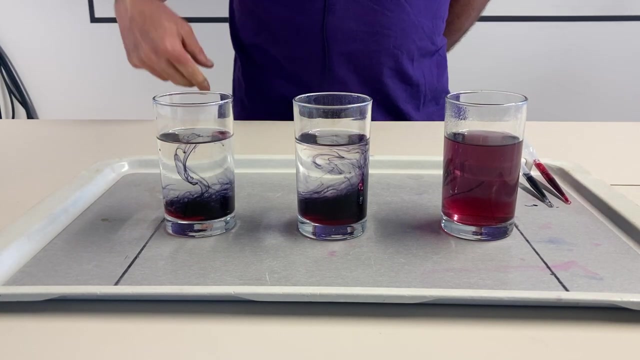 our experiment and you can see in each glass the colors have spread differently. In this glass the colors have not spread very much. In this glass the colors have spread dispersed and mixed quite a bit with the water and in this glass it's basically right in the middle and that shows us.